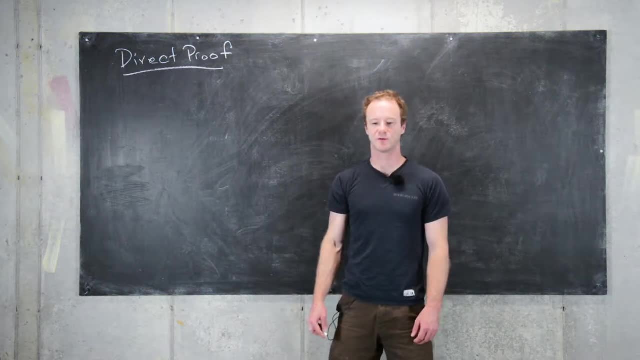 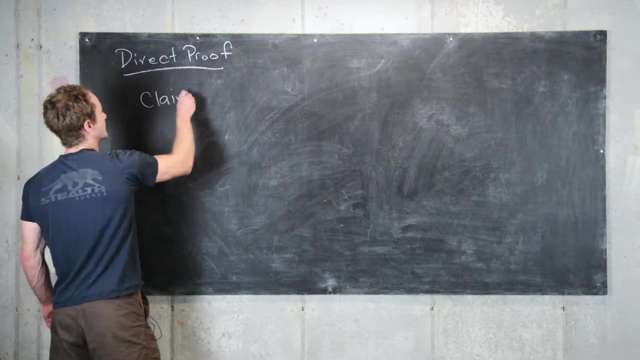 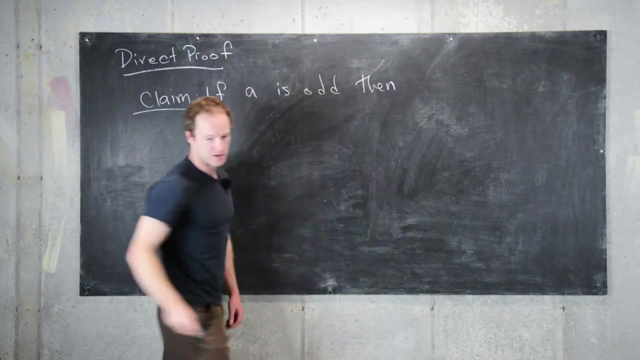 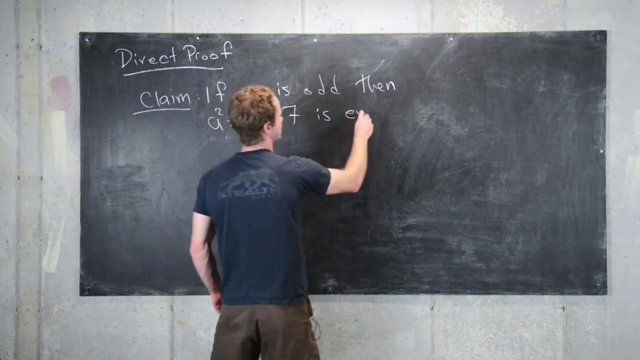 Okay, here we're going to give an example of a statement that's proven with the method of direct proof. So the statement that we're going to look at is the following: So the claim is that if a is odd, then a squared plus 4a plus 7 is even. 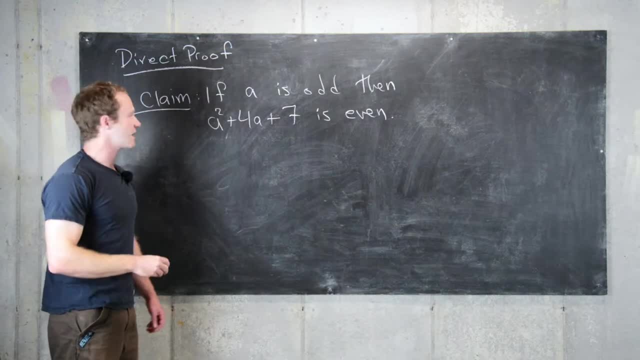 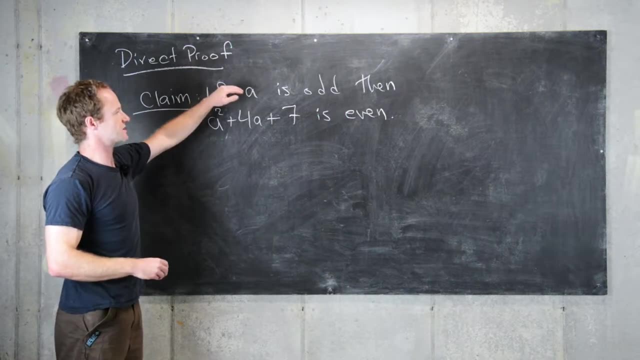 Okay, good. So since we want to use the method of direct proof, there are no tricks in the proof at all. We just start supposing the hypothesis of the proof, do some calculations and end up with the conclusion of the proof. 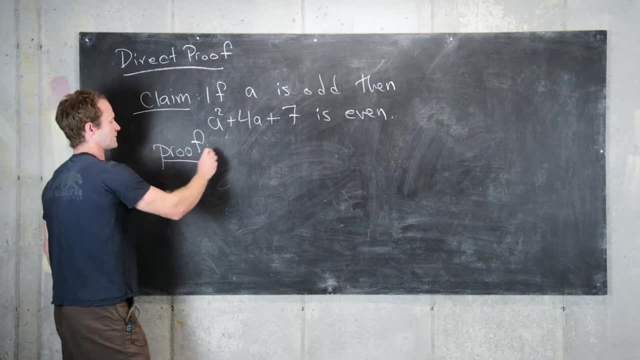 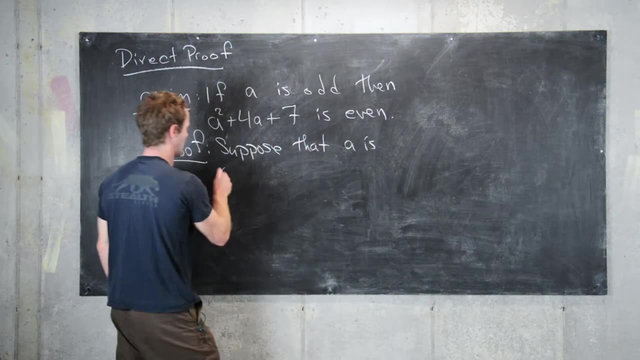 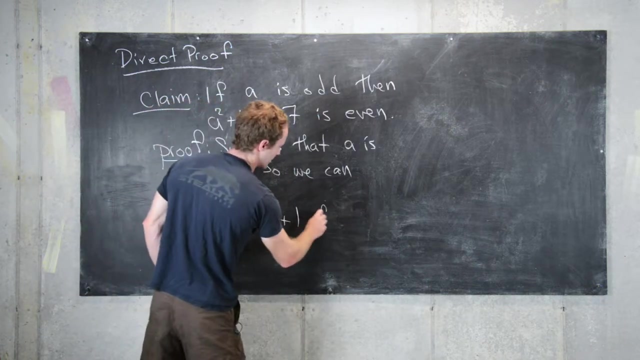 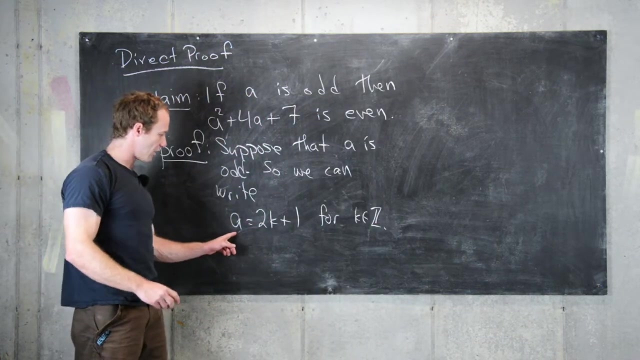 So let's get started. So we want to suppose that a is odd, And so that means that we can write a equals 2k plus 1, for k is some integer. So remember, an odd integer can always be written as one, more than an even integer. 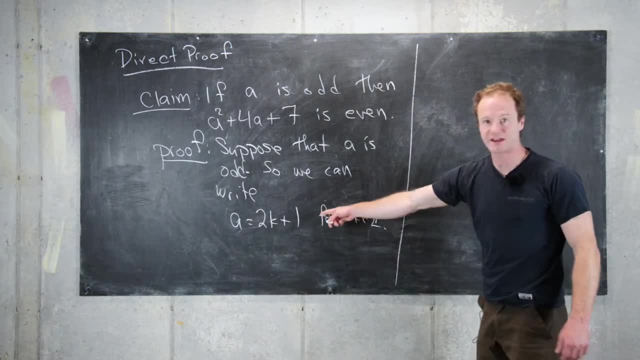 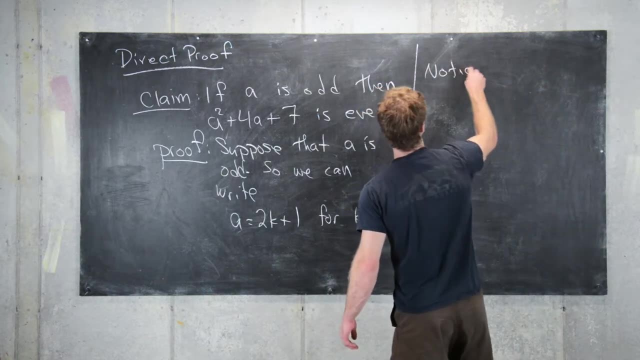 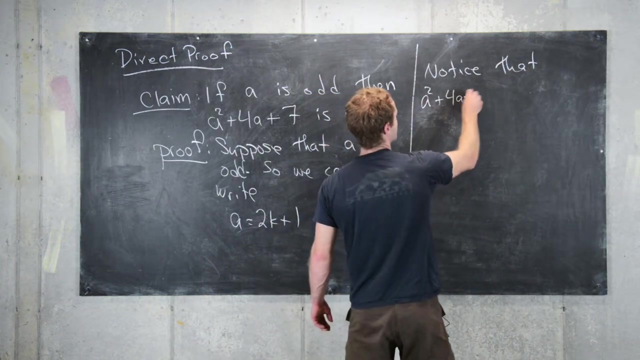 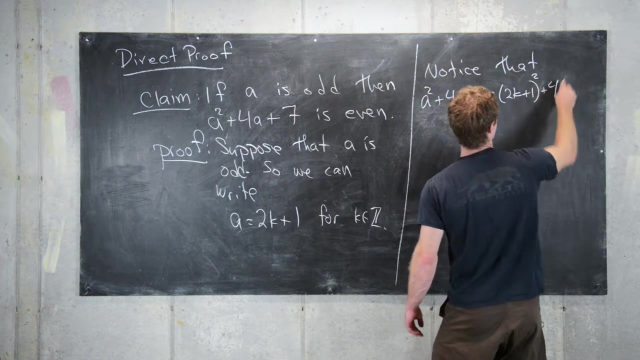 Now that we're set up, we want to plug this version of a into this query Quadratic expression. So now we'll say: notice that a squared plus 4a plus 7 equals 2k plus 1. squared plus 4 times 2k plus 1 plus 7.. 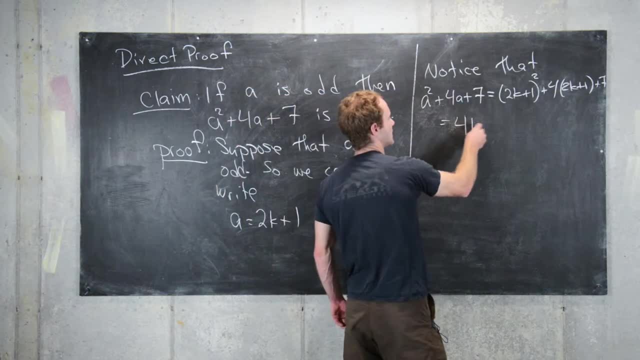 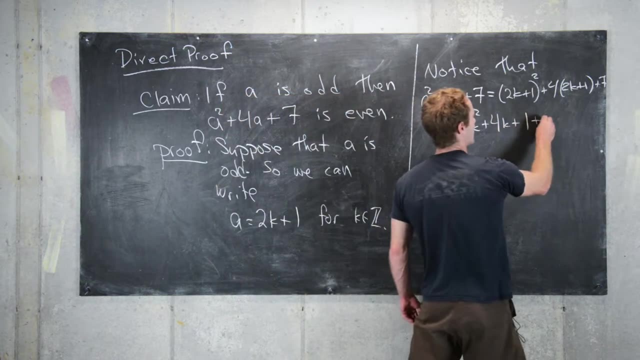 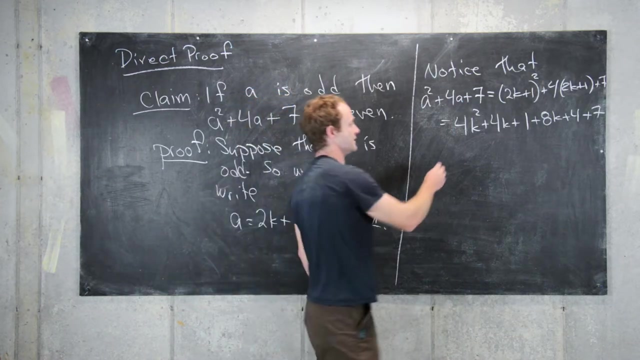 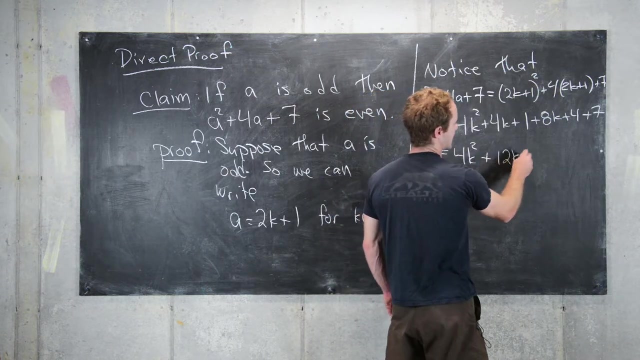 Good, So that's going to give us 4k squared plus 4k plus 1. From squaring that binomial Plus 8k plus 4 plus 7.. Good, So next we can combine like terms So we have 4k squared plus 12k plus 12.. 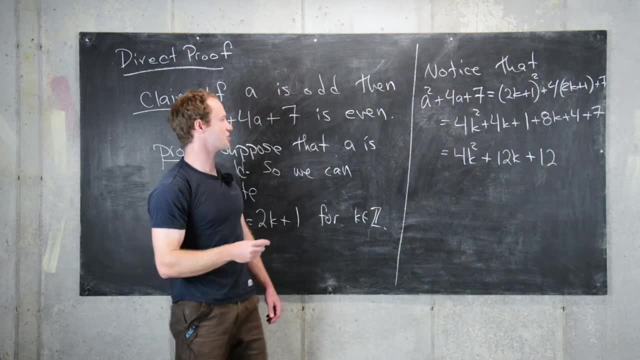 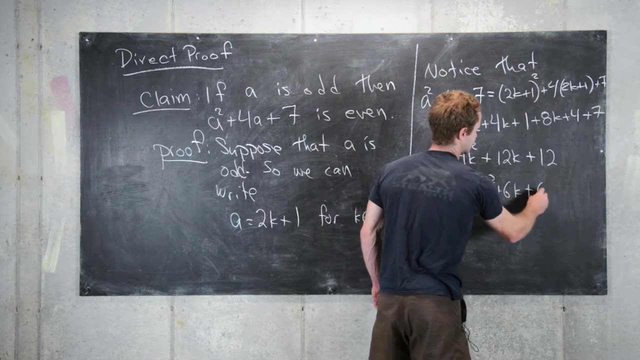 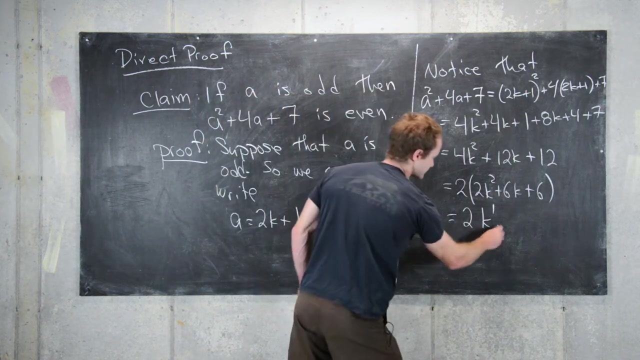 Good. And finally we can factor a 2 out of everything. So this equals 2 times 2k squared plus 6. 6k plus 6,, which equals 2.. And then I'll call all of that k prime, which is even.